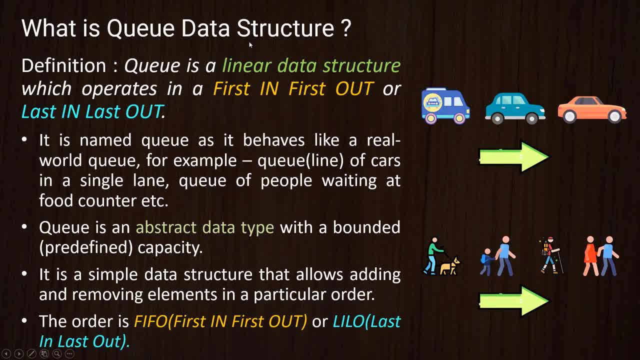 get started. So, starting off with a little bit of theory on Queue Data Structure, what exactly is a Queue Data Structure? The definition would go as follows. So Queue is a linear data structure, just like Stack, and by linear data structure I mean that the data is inserted. 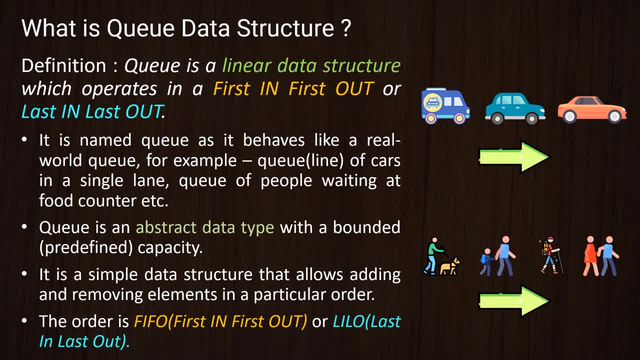 or retrieved in a particular sequential fashion, So it has to be linear. You will understand this term linear more when we actually see the non-linear types also as we move along in this series. Now, this Queue Data Structure operates in first, in first out or last in last out manner. So this is where the Queue 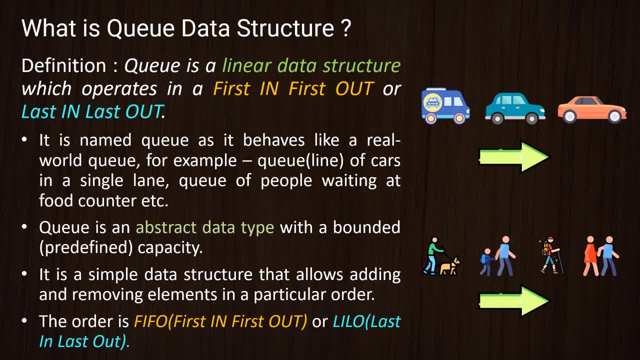 Data Structure is different than Stack. Both Stack and Queue are linear data structures, but Stack operates as first in last out or last in first out. But Queue Data Structure operates as first in first out or last in last out, which means that whichever item or value is stored first in a queue has to come out first. So this is opposite to what happens. 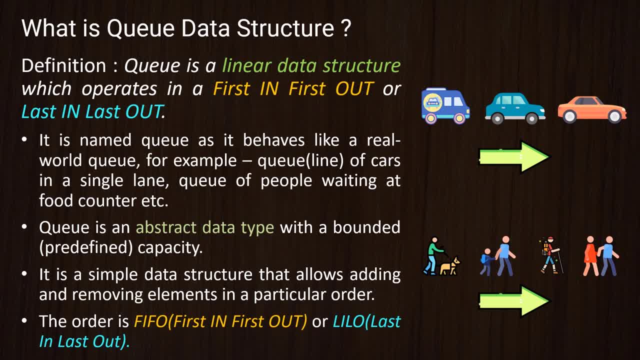 in Stack. Whichever value goes inside a stack comes out last. Now, the reason why it is named as a queue is because it behaves like a real-world queue. So the word queue itself means that there is a line formation and things happen. first come, first serve, For example, a queue. 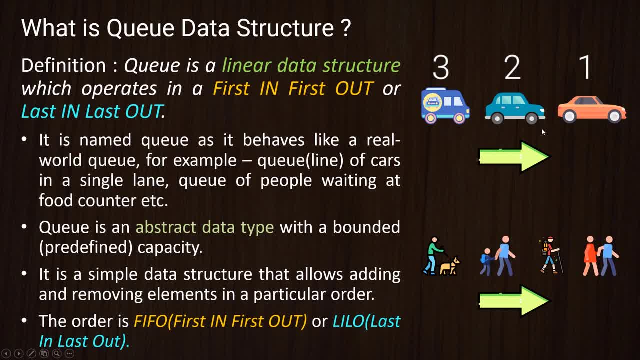 is a single lane road. So, as you can see on the screen over here, if this is a single lane road, the first car to exit would be this orange one which is first in line right, Then the second one and then the third one. Another example would be people walking or 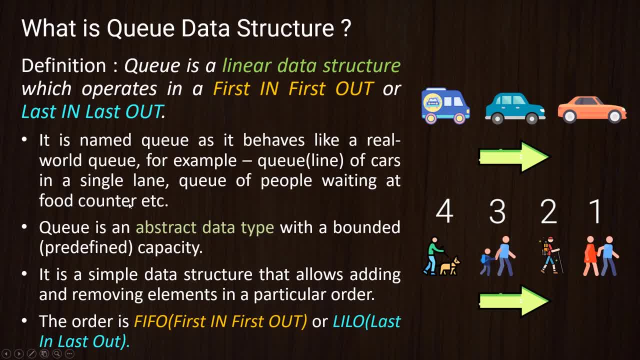 people waiting at a food counter in a particular queue, or people waiting for a doctor's appointment. So there is always a numbering and typically it is first come, first serve, right? So whatever or whoever comes first has to go first. So that's why it is known as a Queue Data Structure. 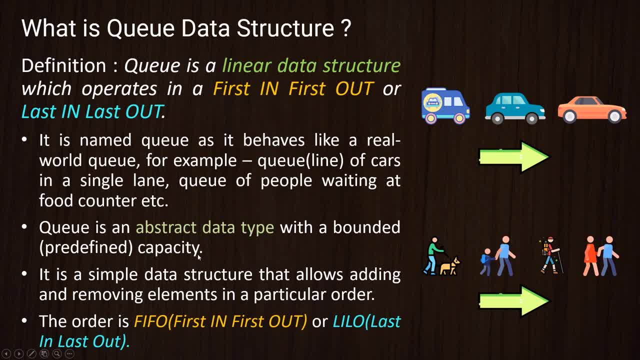 Now again, it is an abstract data type With a bounded or predefined capacity. we've already talked about abstract data types and it's a simple data structure that allows adding and removing elements in a particular order, and this order is first in, first out. Of course, this first in, first out will be more clear. 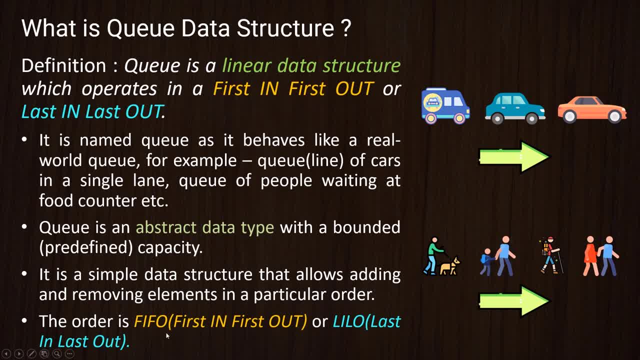 when we actually visually take the diagrammatic representation. So the order is first in, first out, or another way to put it is last in, last out. So this was a little bit of theory on Queue Data Structure and this would give you a very 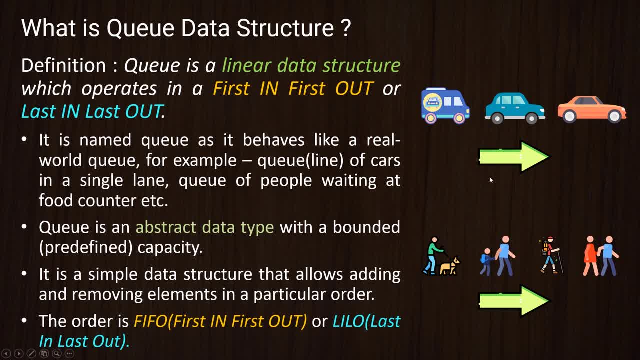 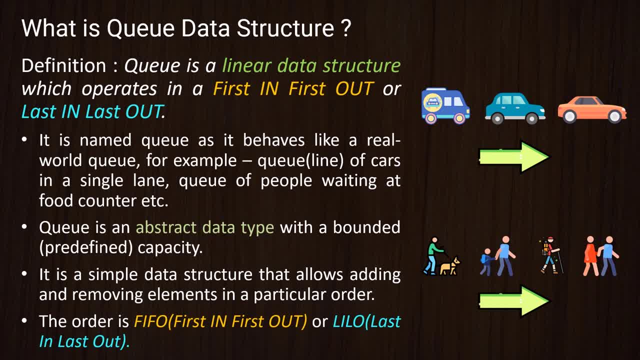 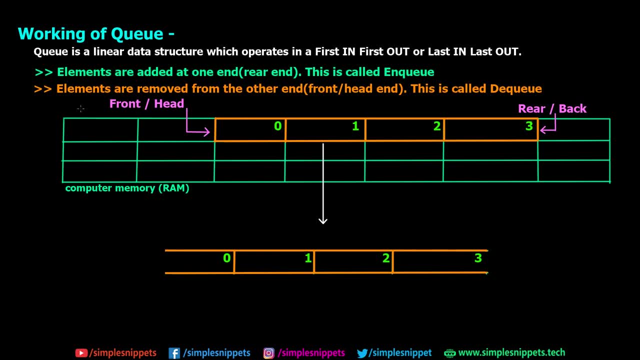 come to the digital blackboard and see what happens behind the scenes when it comes to the digital representation, or the data structure's representation, of a Queue Data Structure. Okay, so, as you can see in the screen, what I have represented over here in this matrix, 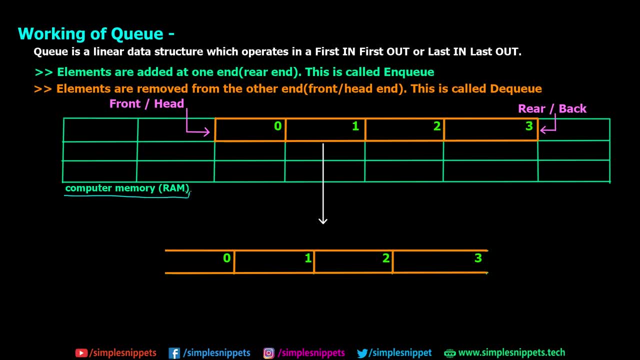 format is basically the computer memory. You can consider this as RAM and we know that each memory location has its unique address. So let's say, this is hash 1000,, this is hash 1001, and so on and so forth. So when you create a Queue Data Structure in the memory, this 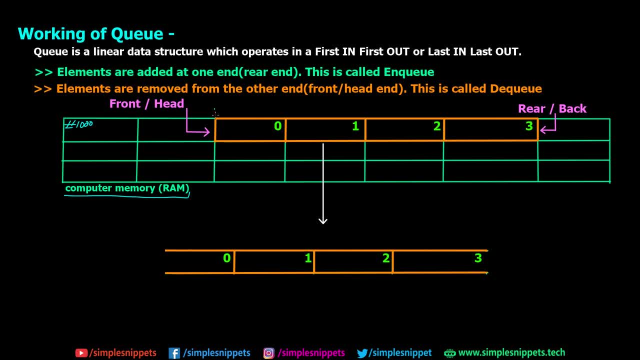 is how it would look like. So what we are currently doing over here is we are saying we want a queue with a size of 4.. You can see 1,, 2,, 3 and 4, the orange rectangular box. So I'm going to say queue of size 4.. Okay, So this registers a queue of size 4. 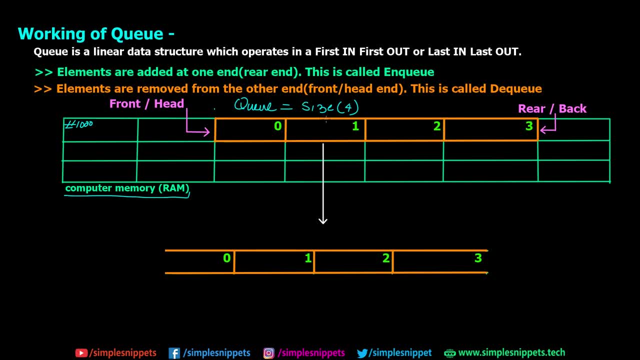 and this is something that visually it would look like Okay in the computer RAM or computer memory. Now, queue always has a start and end, So it is represented by a front or head, rear and back. So basically, there are two important operations when it comes to queue. 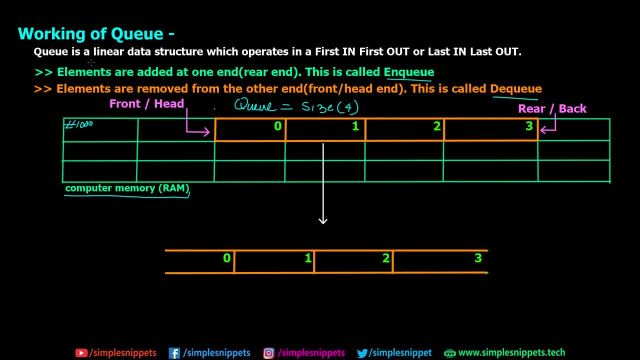 that is called the enqueue operation and dequeue. Okay, now we already know that queue is a linear data structure which operates in first, in first out or last in last out mode. The two more important points to remember are: elements are added at one end. This is called. 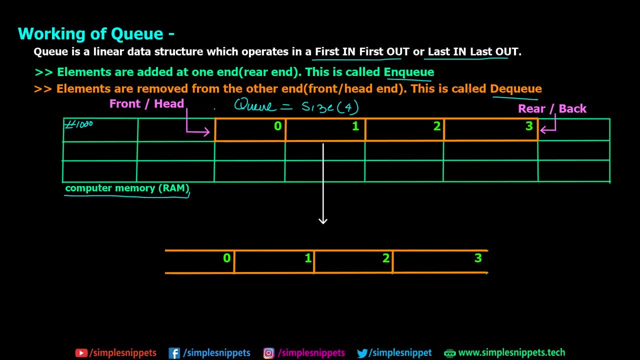 enqueue and elements are removed from other end. This is called dequeue. Now, this is not similar to stack. You know, in stack we had something like this and elements were added also from one end and removed from also from this top. and only right because this 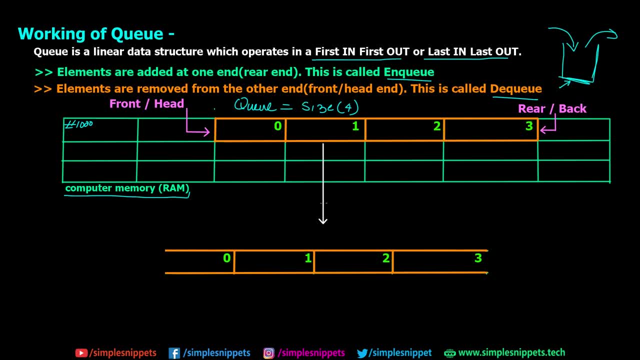 end was closed, But here, if you see so I've represented this entire queue separately over here. Here you can see we have two ends over here. Okay, Now, depending on from where you insert the first value, that would be known as the rear- Okay, elements are added at one. 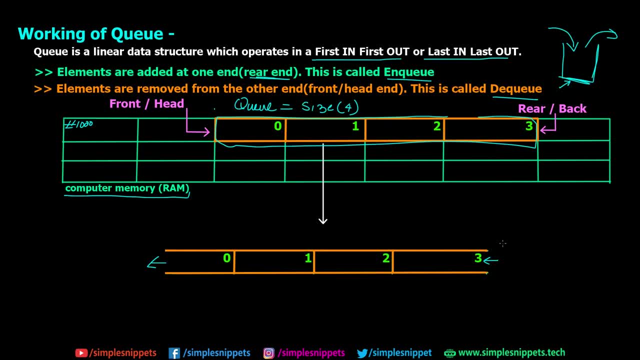 end, which is the rear end. So let's consider this one as rear end- over here. So elements would be added from over here And they would be removed from over here. So elements would be added from over here And they would be removed from the other end, because the other end is also open ended. 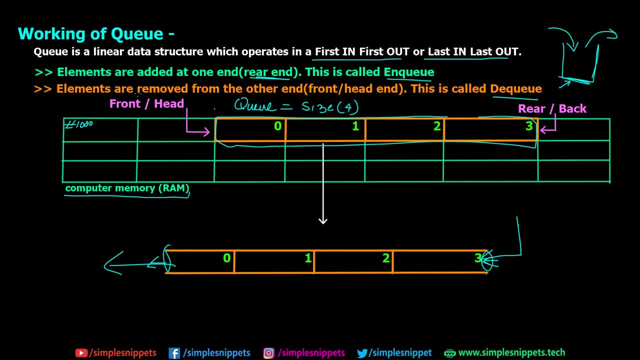 right. So this is also open and this is also open. So when they're removed, they are removed from other end, which is the front end. So this is the front and this is the rear. Okay, So when it is inserted, when the value is inserted at rear end, it is called enqueue. 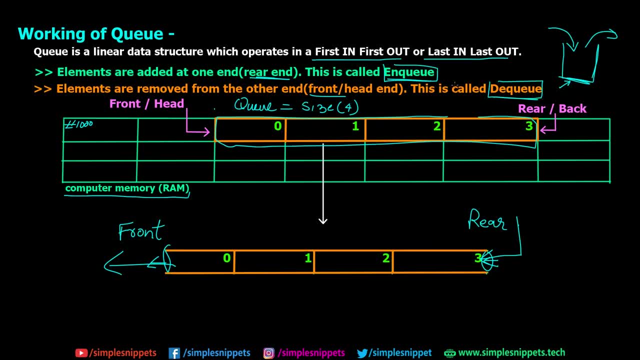 Remember this term, and whenever it is removed it is called dequeue. Okay, fair enough. So let's say, if I insert a value five, it would be inserted over here and it would be coming directly over here. Okay, at the start of the front. that is the front end. So let's. 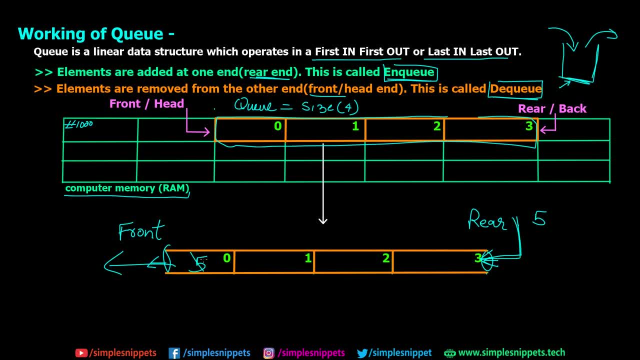 say that is the front end side And whenever it is, it will be removed. this would be made zero or null or whatever, and it will be removed from over here, Okay, Similarly, when you perform two or three enqueue operations, let's say, after five I insert one, So one would. 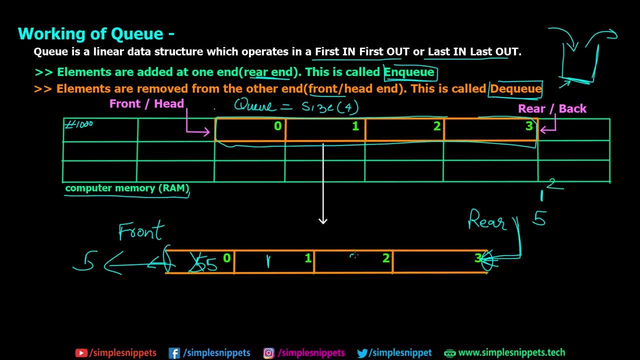 come over here, five would be here. If I insert two, it would come over here, and so on and so forth. Okay, So I hope you can visually imagine how a queue would be in the memory. Okay, this is how the operations would go like, But now let's see more in detail how. 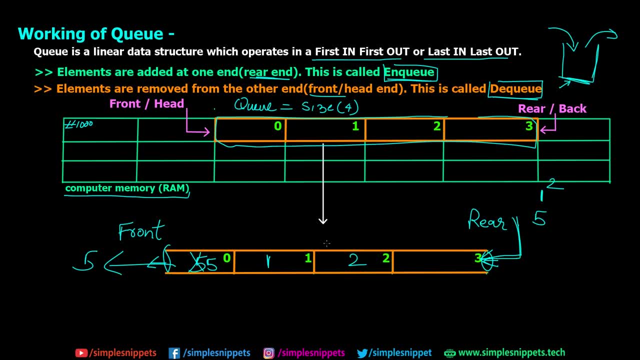 the operations would look like. That is the actual standard queue operations And we'll also try to understand the algorithm, that is, the pseudocode, and how the steps would look like when you perform these different standard operations. So we have five standard operations over here We can actually have. 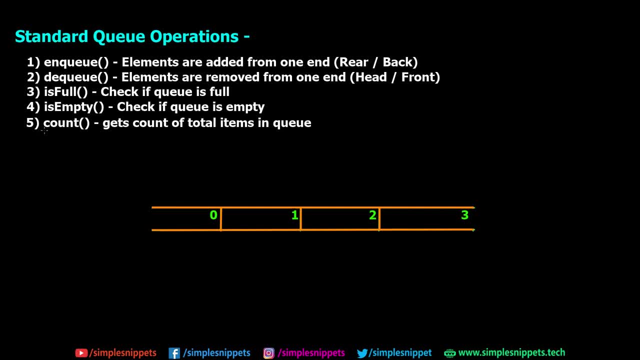 a few more, that is, peak and change, but those are not really very relevant over here. We are going to be implementing these five different operations. The first one is enqueue, which means elements are added from one end. So let's say this is the rear and this is the. 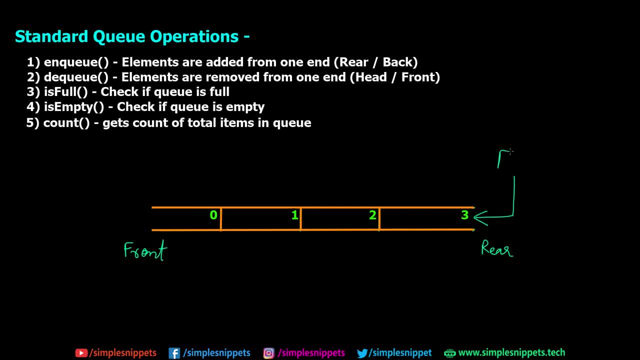 front. Okay, So from here when we add things, it would be enqueue. Dequeue is elements are removed from one end. We just saw that. So when things would be removed over here, it would be dequeue. The third one is isFull. Now, as the name suggests, we are going to check if the queue 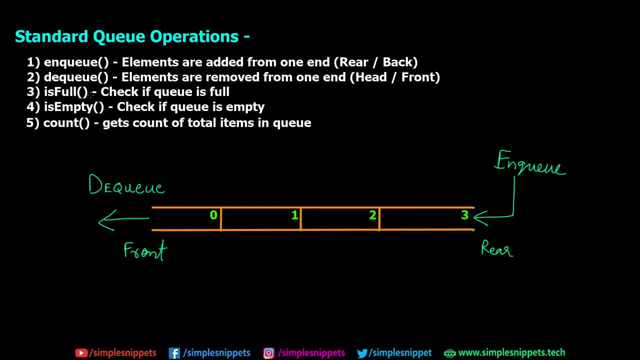 is full or not. Now, the reason why I have opening and closing parentheses is when we actually implement these operations in terms of implementation, in terms of a program, we will write different functions for them. Okay, So that's why I've already denoted 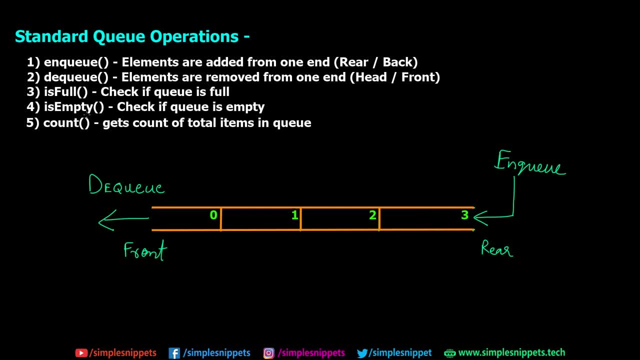 them in opening and closing round brackets. The next thing we are going to do is we are going to check for the empty queue. empty and empty. The question is: is empty as the name suggests? if the queue is empty, let's say there's nothing inside. then we say it's. 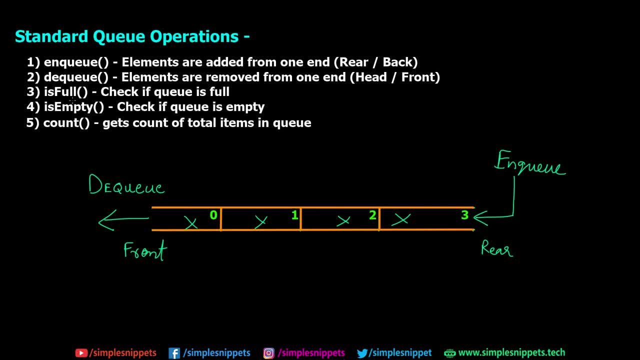 empty. Of course, we will see what are the different conditions in a minute and how to actually check for these different conditions. And lastly, we have the count, that is, how many values are actually there inside the queue. Now you are. the queue size is four. 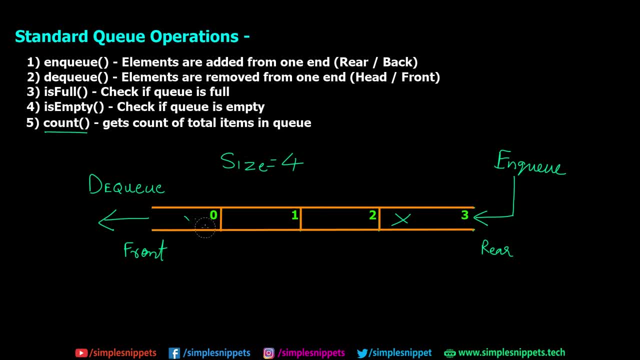 but let's say there are only two values inside, Right? Let's say we have five and six, So currently the count is going to be two. Okay, So the count keeps on changing depending upon the enqueue. Okay, So the count keeps on changing depending upon the enqueue. Now. 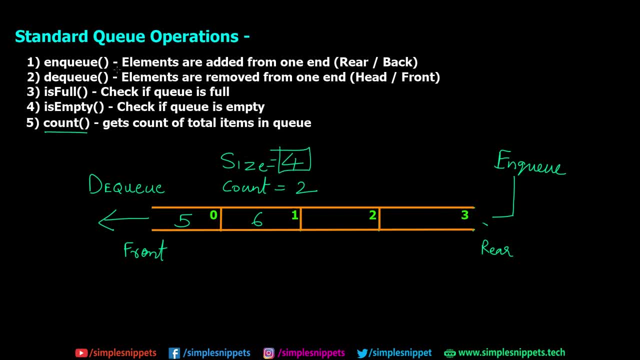 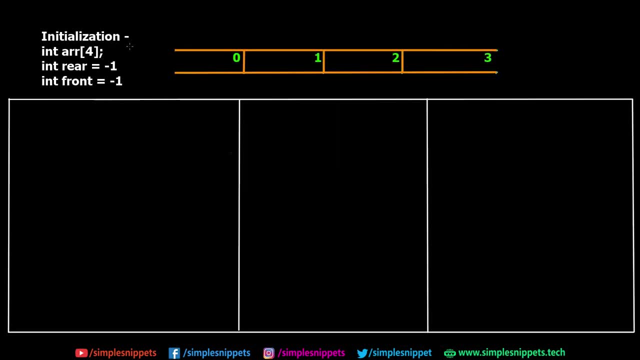 and DQ operations where the size is going to be constant. Okay, Now let's see the different algorithms behind these individual operations. Okay, So before we start off with the different operations, we have to do a particular initialization Now, when we are going to be. 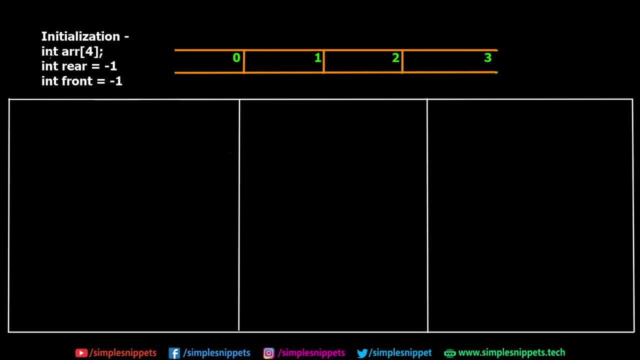 implementing this queue. in the next part, that is, in the program for implementing queue, we are going to be using arrays. Okay, Now there are different ways in which you can actually implement queue or stack. also, like you can do it with another data sector, which is known as linked. 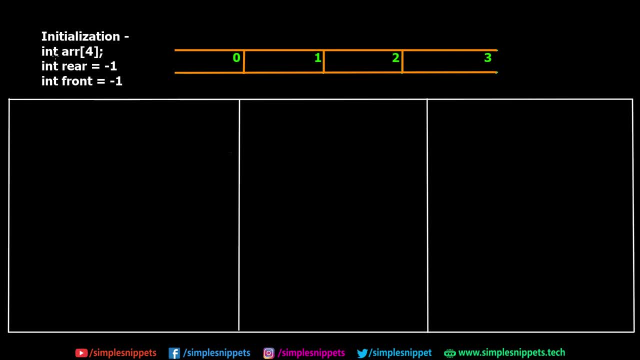 list. But since we haven't yet studied that, we're going to go the simple route. We are going to use arrays to implement queue, just like we used array to implement stack, And here the initialization is as follows. So the first thing we are going to do is we're going to say int, ARR. 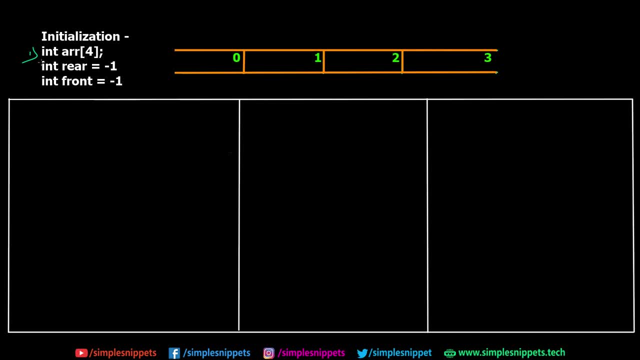 of four, which means that our array size is four and it is an integer type array. Okay, So this is that representation right now, over here. Now, since we know that elements are added from one end- that is, the rear end- and they are removed from another end, we need to have two different. 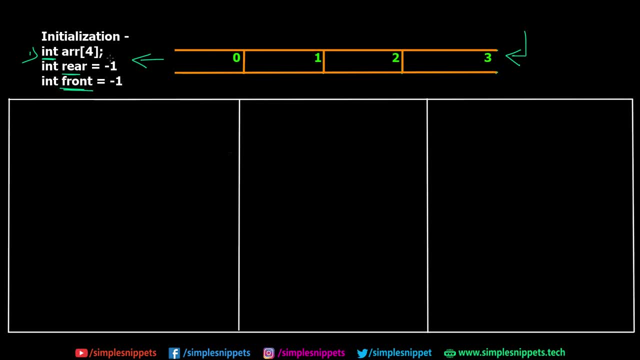 individual variables which are going to be keeping a track of the index positions In stack. we only had one end right, We only had the top, which was keeping a track of the top of the stack. but in queue you can see that since elements are added at one end and removed at another, 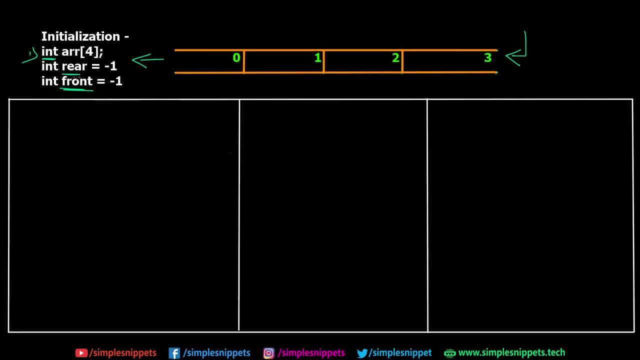 we have to keep a track of both the ends Now. things would be more clear when we move ahead and see the actual algorithm, But right now, just keep in mind that initially what we will do is we will say rear end front equals to minus one. Okay, Now remember, we are going to have a 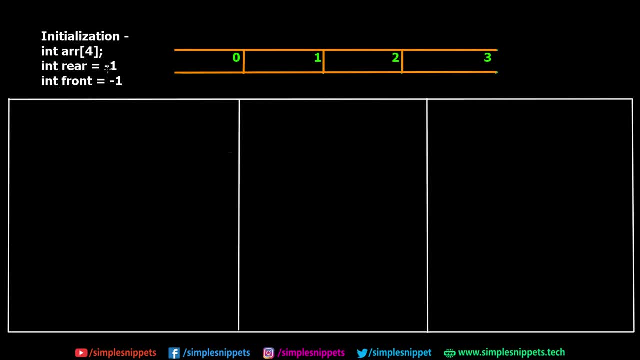 number that these are not pointers. These are simple variables which are just keeping a track of this index location. So minus one would be somewhere over here, which is not exactly a valid index location. right In arrays, index start from zero, So right now. 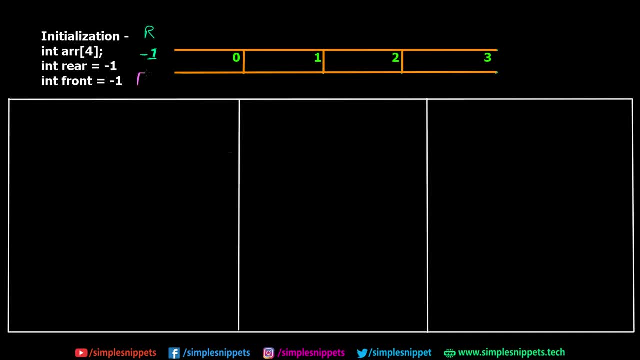 let's say, for rear I'm going to say R and for front I'll say F. So this is the initial part that we have to do when you create a queue data structure. And now let's see the individual operations. So the first operation is is empty. Okay, Now here we simply check. 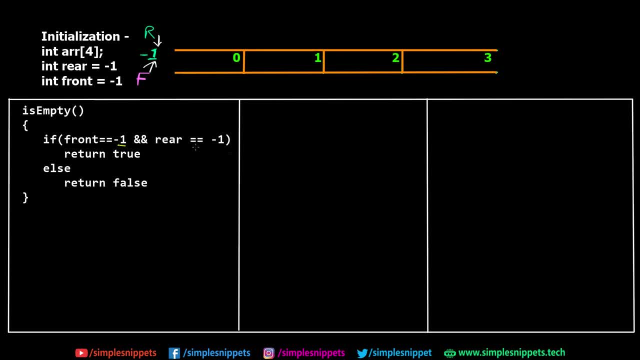 if the front value is equal- equal to minus one and the rear value is equal- equal to minus one, Because when the initialization happens, front and rear are going to be set to minus one right, Which means that nothing is going to be there in our array. that is nothing is going. 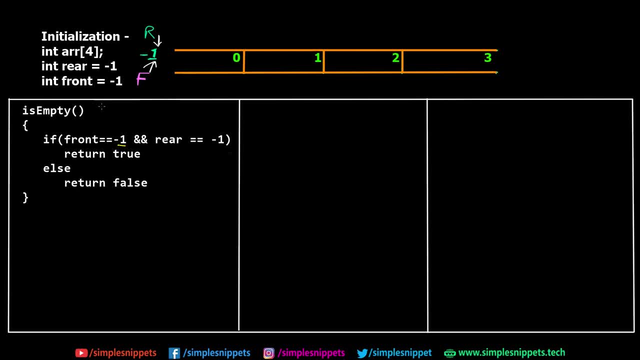 to be there in our queue, So it will return true, And this would indicate that our queue is empty. Simple enough. This seems very basic, right? Let's see another operation. that is is full. Now in is full. what we're checking for is if the rear equal equal to size of. 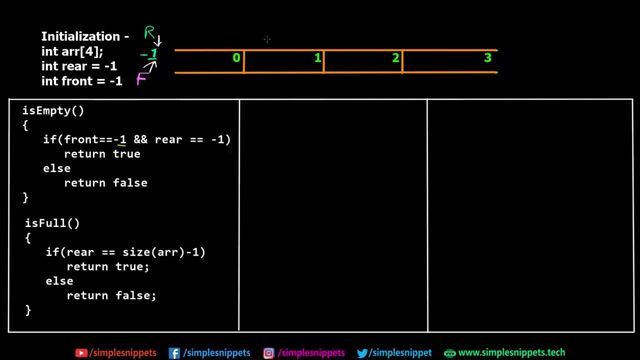 minus one return true. now what happens is when you add a new value, the rear pointer has to be incremented or the rear variable has to be incremented to keep a track. So basically, currently you can see rear is pointing minus one. So let's say I perform an NQ operation. 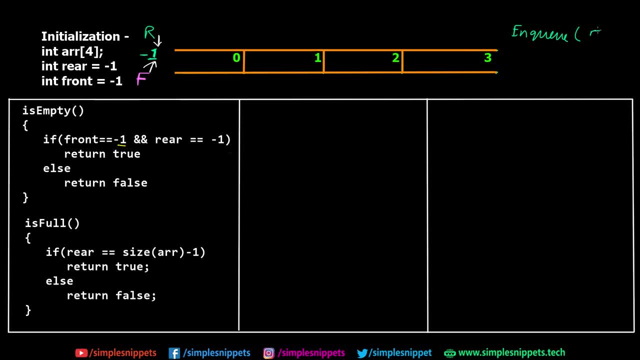 I say enque And I insert a value, five. Okay, So this five would be stored over here, right? So it would be completely inserted and taken to the front of the queue. So this is the front end, right, this is front and this is rear. so whenever an enqueue operation happens, we have to say: 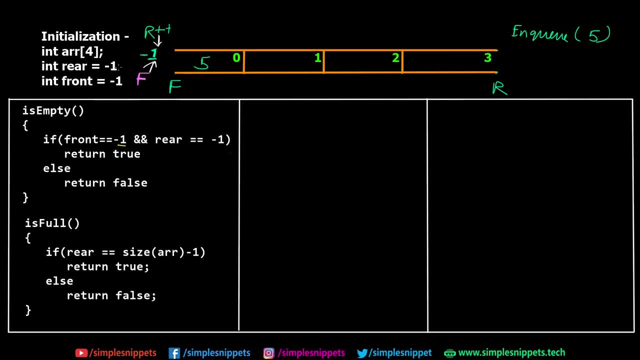 rear plus plus. okay, so currently rear is minus 1, so now the rear would be pointing this one also for the first time. that is when the first value is inserted. we also have to say f plus plus, which means that the f variable or front value will also point to the first location. 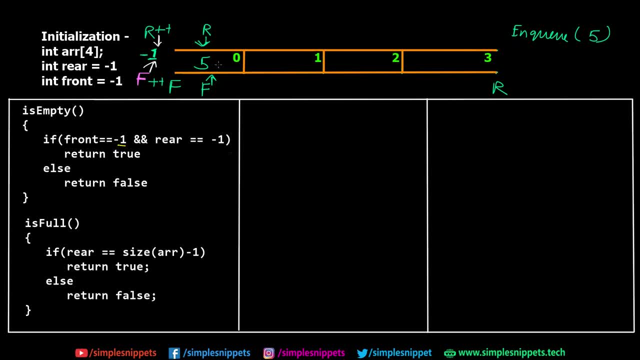 because when the first time the first value is inserted in the queue, the rear and the front is basically one and the same right. whenever there is one more enqueue operation happening- let's say i enqueue 3 and 3 is coming over here- now the front and rear are different. 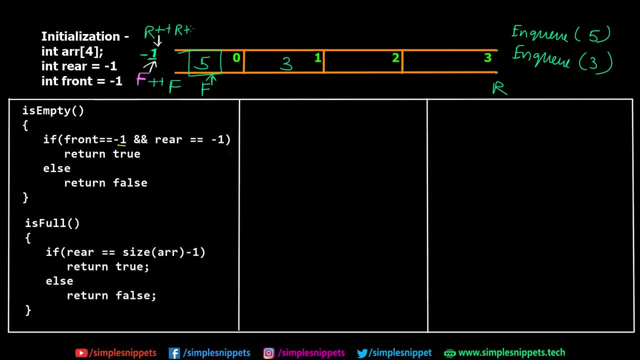 right now. the rear would be again plus plus and rear would be pointing to this location, that is 1. so from minus 1, first enqueue operation, we did r plus plus and f plus plus. so r and f become perfect 0 and 0. right, they were pointing 0 and 0. for the second nq operation, only r is going to be. 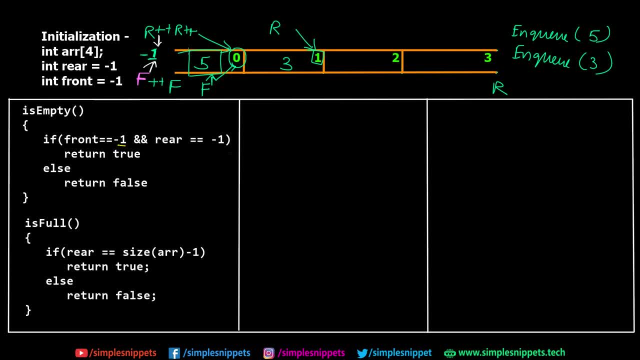 incremented because now the front and rear are different. the value at the front is 5, the value at the rear is 3, right? so there are two different ends now. i hope you're understanding this. so that's why, when you're checking for is full, we only check for the rear value and we check that. 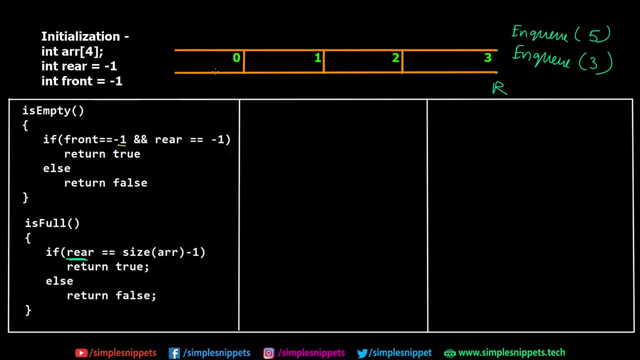 if rear equal equal to size of arr minus 1- now here you can see- the size is 4, size equal to 4. if you perform four nq operations, the rear value r would have number 3 as stored in it, which is 1 less than 4. so that's why you have to check: if rear equal equal to size of arr minus 1, okay, and 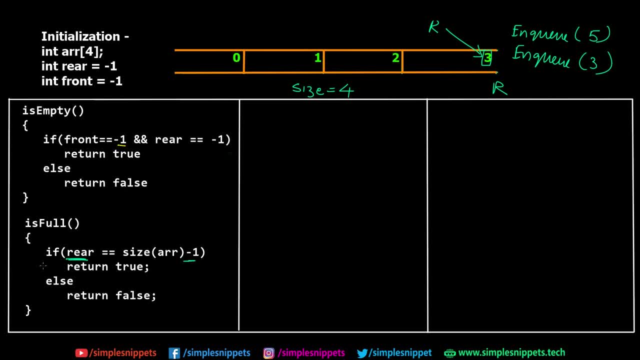 if it is true, you have to say it is full. so this is the is full operation. i hope you have understood this, and things will get more clear when we actually see the nq and dq operation also. so let's see the nq and dq operation. okay, so this is the nq operation. now it says that first we have: 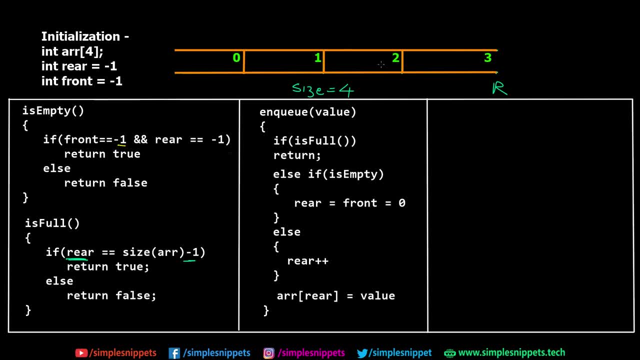 to check if the queue is full or not. obviously, you cannot add more values inside the queue if the queue is entirely full, right? so the first thing that you have to do is you have to check if the queue is full. now we just saw the algorithm for is full. so this is the pseudocode. now, if it is full, obviously. 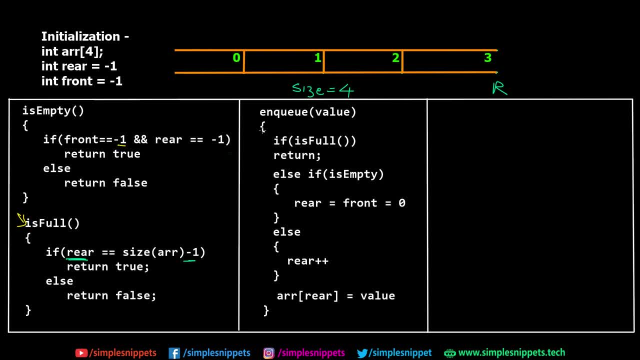 you have to not proceed ahead, you have to return from over here, you have to exit this method or exit this operation, and you have to print a message that queue is full or queue overflow or something like that. right, so if this condition is not true, you have to check for one more condition. 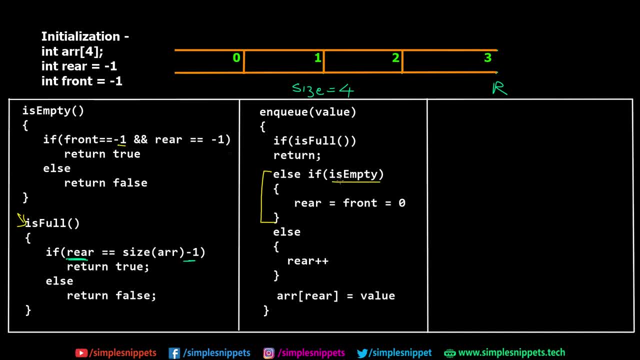 which is if is empty. now, the reason why i have to check for this is empty is because when the queue is empty, remember that the rear pointer and the f pointer- that is, front pointer- and i'm calling it pointer, but it is not exactly a pointer, it's a variable- is going to be storing a value of minus. 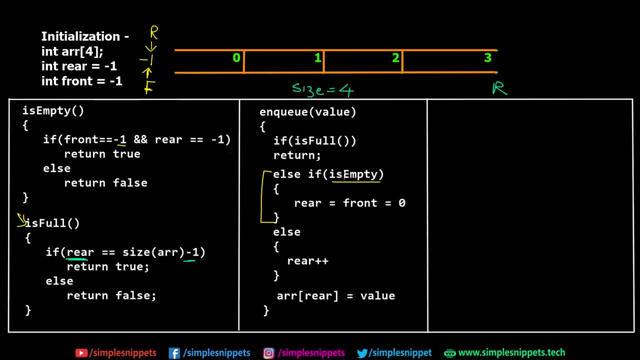 one which is not a valid index location. so whenever it is empty, remember we are checking for front equal equal to minus one and rear equal equal to minus one. so when you're performing an nq operation, if it is empty, the first thing that we have to do is we have to check for the front equal equal to. 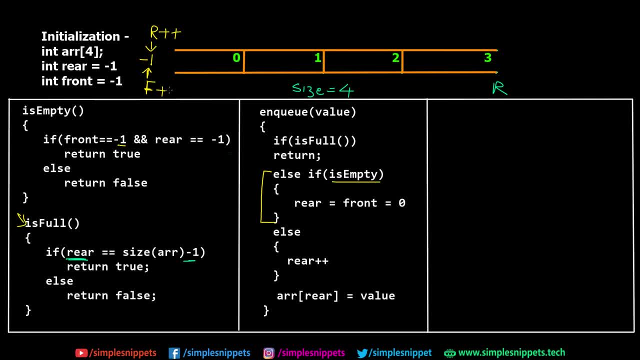 we have to do is we have to increment this rear pointer and front pointer by plus, plus, so that it points to or it stores a new value of the index location of zero. okay, and the third condition is, if there is some already existing value, then you have to just do rear plus plus. so you have to. 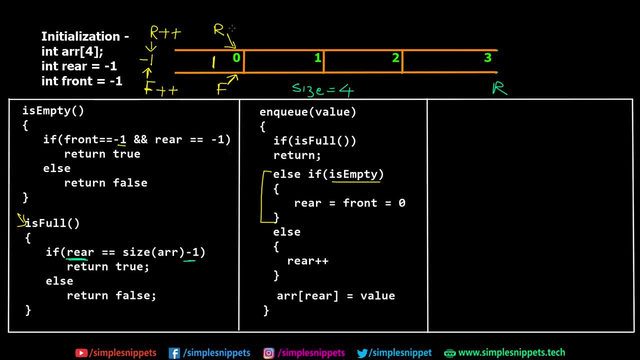 increment this. let's say we already had some value over here one. then you only had to increment this r plus plus, right, and at the end of this function you actually enqueue the value. okay, so if i say nq, so you have to pass some argument in the nq function when you actually 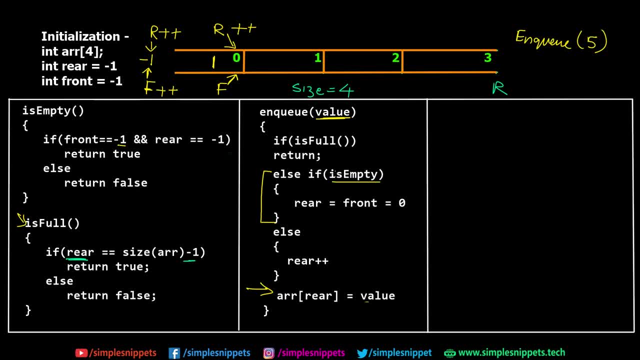 implement it if i say nq, phi, and let's say, if our q is empty for the starters. so what will happen? r will get plus plus, f will get plus plus and they will both store the new index value of zero. this else will not be executed. because this else if got executed, because for the first time the 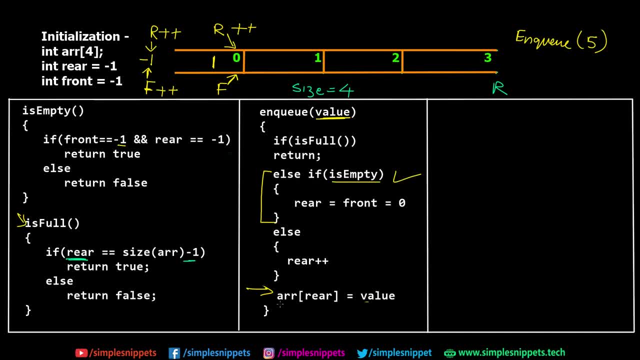 q was empty, right. so this part got executed and at the end we are saying arr of real, which means that arr of zero, because r has now become zero, right, r is storing zero. at this point we store the value, and that is phi. so i'm going to store phi over here. okay, let's do one more, nq. 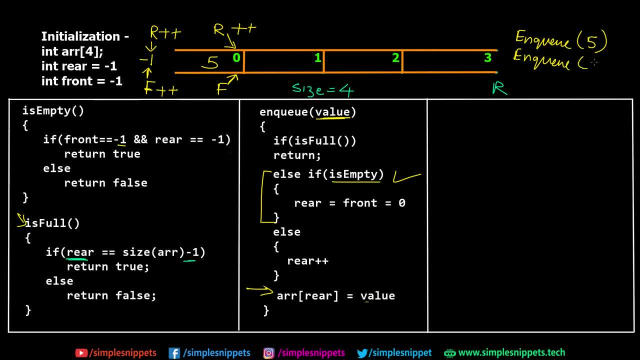 so i'm going to say e, n, q, u, e, u, e, and here i'm going to say three. so now again, what will happen? we will pass three over here. we will check if is full. obviously it is not full because the rear is not equal to size of arr minus one. what is the value currently? that is, rear storing zero. 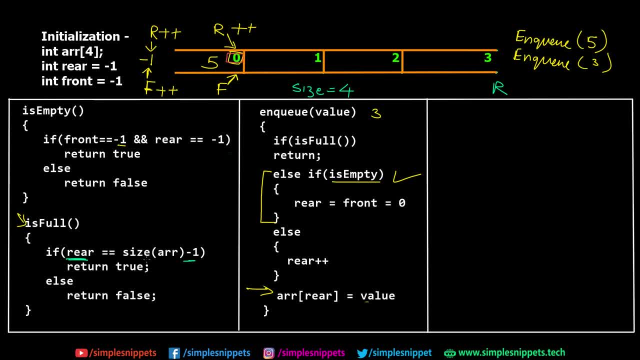 right. so this is the value now. zero is not equal, equal to the size of arr minus one, that is, it is not equal to three. zero not equal to three, right. so obviously the q is not full, which means that this part, the if part, is not gonna get executed. right, let's move on to the else if part now here. 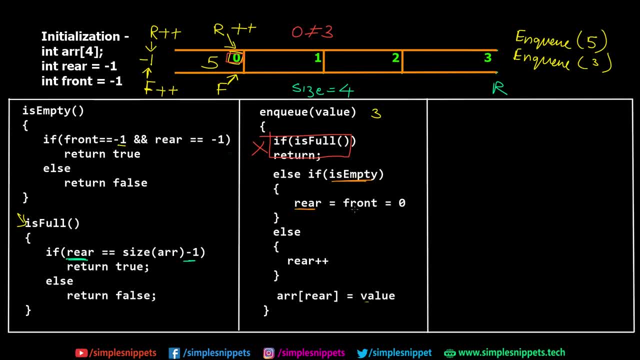 we are checking for is empty. here we are checking rear equal to front, equal to zero, but we know that in is empty. we check if the front or rear is equal, equal to minus one. now, after performing the flying part, where the front equals to zero, we check if the back or rear equals to minus one. after performing the 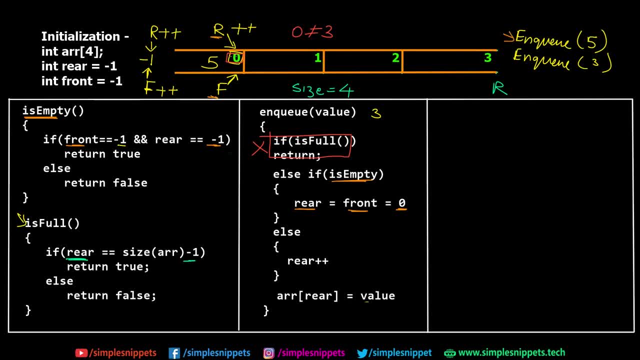 first nq operation, the rear and the front has become zero, which means that this will return false. so it is not empty, right? so even this part else, if part is not gonna get executed, which means essentially the last else part is going to be executed and the else part says rear plus, plus. 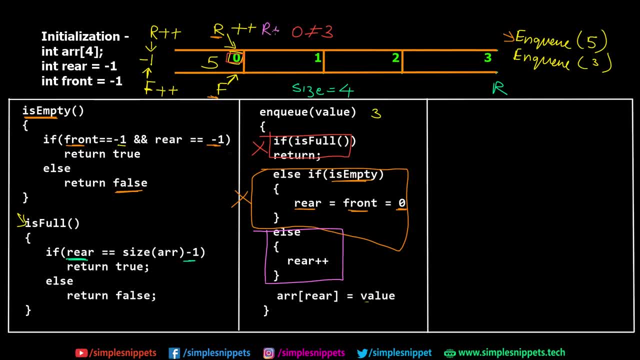 so r plus. so we will have r plus plus, and now the r is going to store one. once we increment the r plus plus, we are saying arr of rear equals to value. so then this new value three that we passed is going to be stored at arr of one. so three goes over here. okay, so f is currently zero, r is 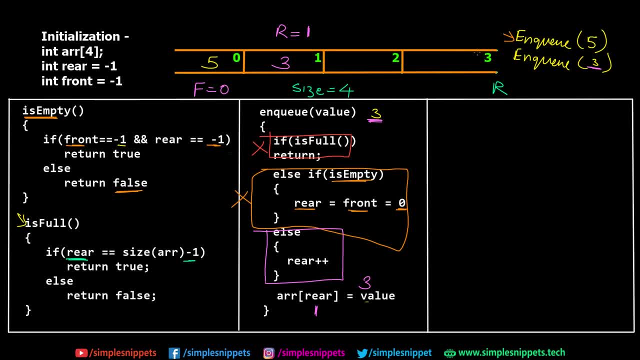 currently one. let's perform one last nq operation. so i'm going to say nq two. so the value that we are passing in the nq operation is two. again, it is going to check is full. the is full condition is if rear equal equal to size of arr minus one rear over here is one. 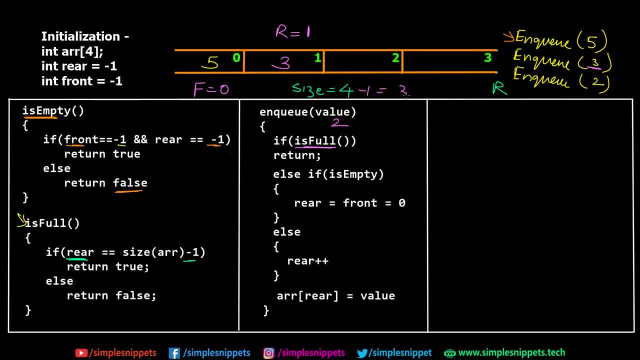 is one equal to four minus one, which is three. no right, one is not equal to three. so this means the first. if is not going to get executed, let's see what happens in. else, if here we are checking, is it empty? is the entire q empty? for that we need to check for this part, that is, if front equal, equal. 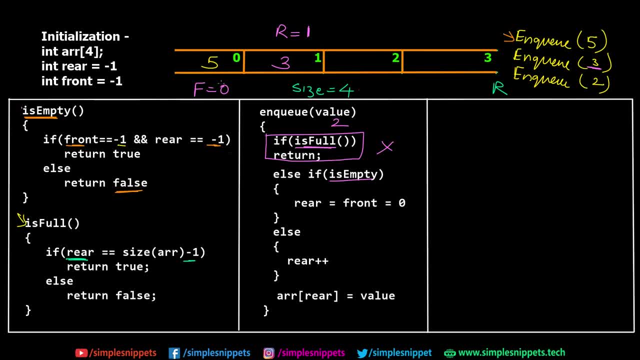 to minus one and rear equal equal to minus one. but now we know that f equals to zero and r equals to one, so your false is going to be returned, which means that else if is also not going to get executed. so, lastly, only the else part is left. so here what is happening? rear plus plus, so now r equals to: 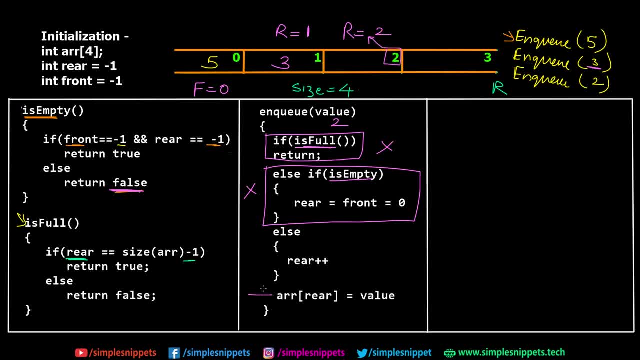 two, so this index location is stored in the rear. and lastly, we are saying arr of rear equals to value, so now we are adding two at this location which is pointed by rear variable. okay, so this was the complete nq operation. i hope you've understood. we performed three different nq. 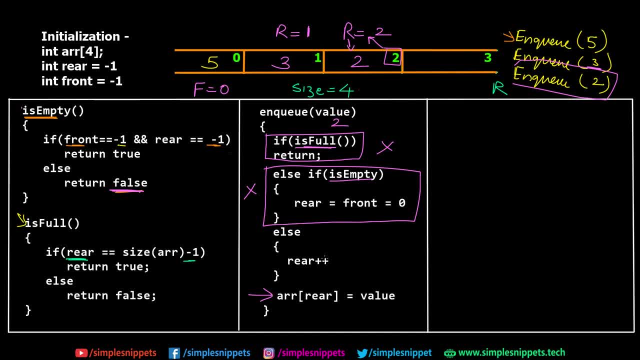 operations, and this is basically the pseudocode. this is not the exact syntax, but this is pretty similar of how it would look like in a c plus plus program also. okay, so now let's see the last operation, that is, the dq operation. now, in the dq operation, what we? 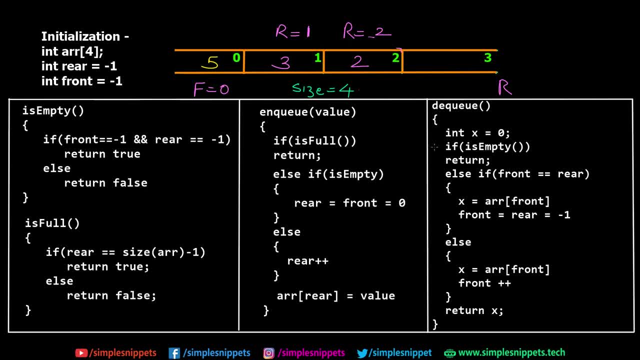 have to do is, first of all, obviously we'll have to check if the q is empty or not, right? if the q is empty, obviously we cannot remove more values. right, because it is already empty. what are we going to remove, right? so here, what i'm creating is i'm creating a temporary int x variable. i'll tell. 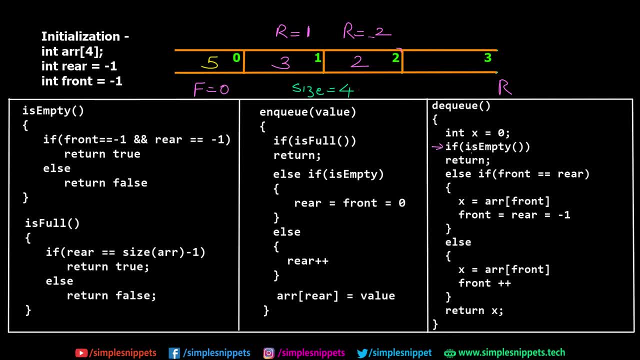 you why we need that step two. we are checking if the q is empty. now in is empty. we check if front is equal- equal to minus one, and rear is equal, equal to minus one. obviously, since we have already performed three nq operations, you can see we have five, three and two. so the front is storing zero and 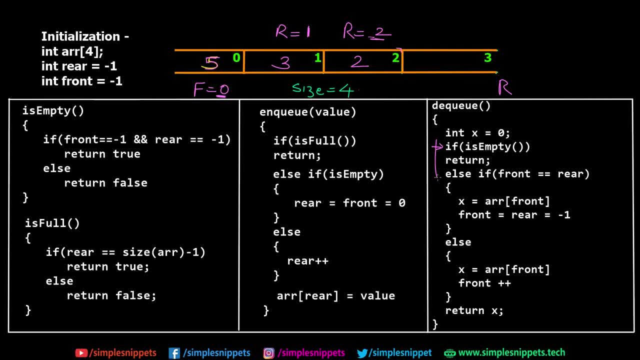 rear is storing two right, which means it it is definitely not empty. so this if part is not going to get executed. let's see what happens for the else if part. now. in the else if part i have a condition which says if front equal, equal to rear. so when will this condition ever happen, or when? 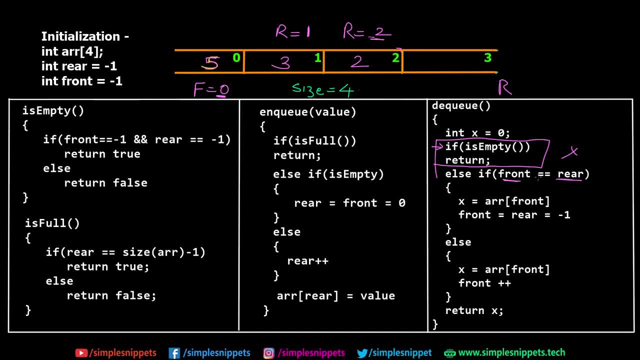 will this condition ever be true? this condition will ever be true because if front is equal to, if the value stored inside f is equal to value stored inside rear. now remember, this happened for the first time when we inserted one value, when r was also equal to zero and f was also equal to. 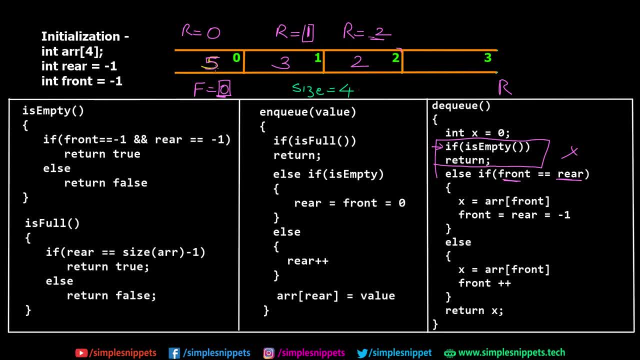 zero, and this only happens when there is only one single element in the q right, whenever f and r are going to be equal and not equal to minus one, because we have denoted minus one as an invalid state, invalid index, which which denotes empty, other than minus one if r and 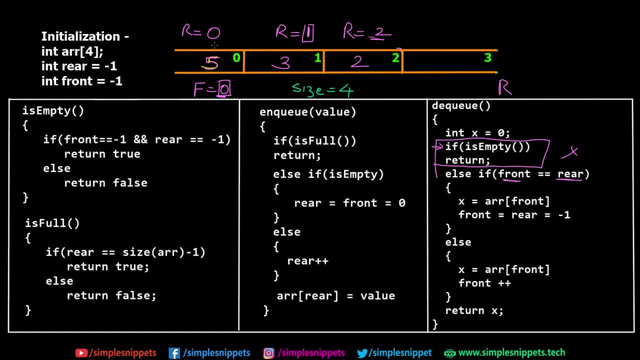 f are going to be equal, it would indicate that there is only one value in the q, right. so in that case, what i'm doing over here is i have to remove that one single value. it would mean that there is one value left and dq always removes that value, right. so i'm storing that value, i'm going, i'm. 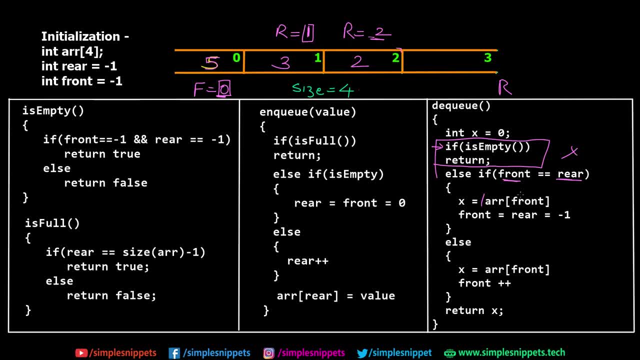 going to say arr of front. so whatever the index location is, i'm taking the value at that index location, storing it in x variable that i created on top over. here i'm saying front equal to rear. the reason why i'm doing this is because i know that when front and rear are equal to each other, 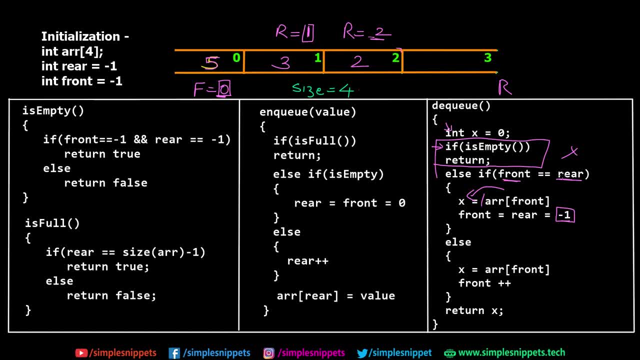 it would mean that there is only one item in the q and when i dq that i have to make front and rear as minus one. i have to make the q empty right, and the condition for empty q is minus one. so that's why i do that over here and then if else, if is going to be executed, this else part will not be. 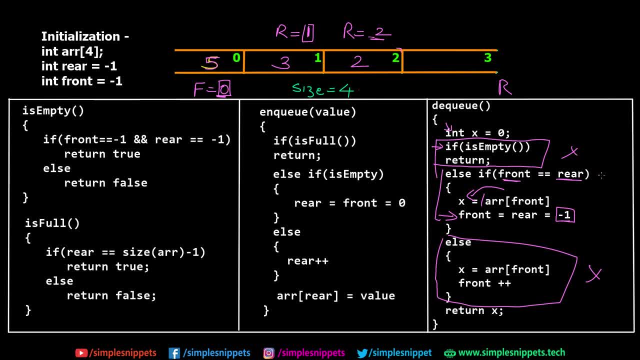 executed right, this part will not be executed. so from else, if we will directly jump to the last line of code, which is return x, so x has stored the last value and i'm popping that off or i'm dqing it, i'm removing it from the q right. so 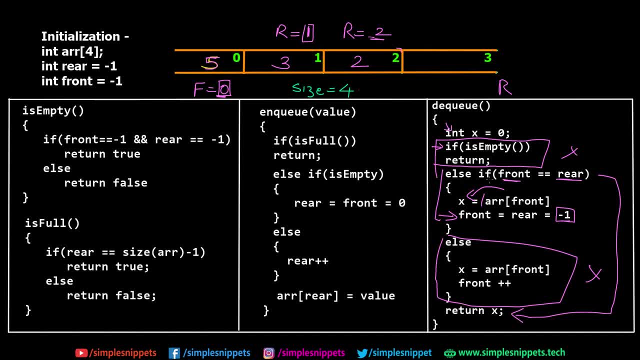 that's why i have to return that value. so this condition, that is, the else if condition, is only for one special case, that is, when there is only one single value in the q. okay, now let's see the last condition, that is the else condition. so the else condition is for when there are some values. 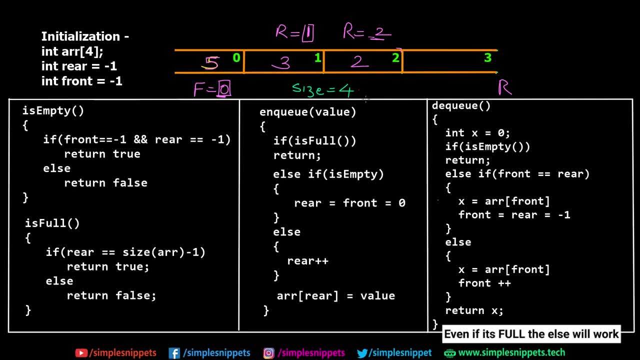 more than one, but not full. so the q is not full, but it also doesn't have one single value. it has multiple values, just like the current q is having three values, right? so in that case what we do is we say x equals to arr of front. 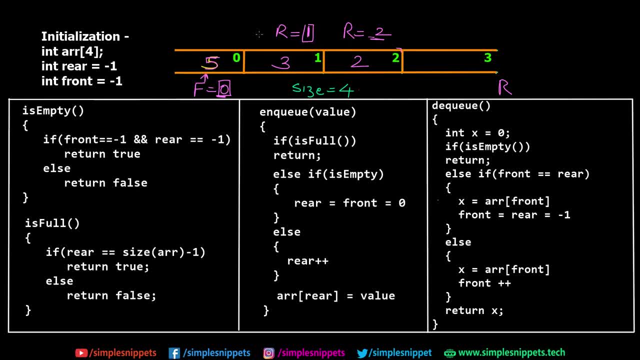 because the front value has to be removed right, not the rear value. inserting is going to happen from rear, rear end, and removal is going to happen from front end. so i'm going to say: arr of front equals to x, so here currently f is equals to zero, so the value at zero index is five. so that i'm 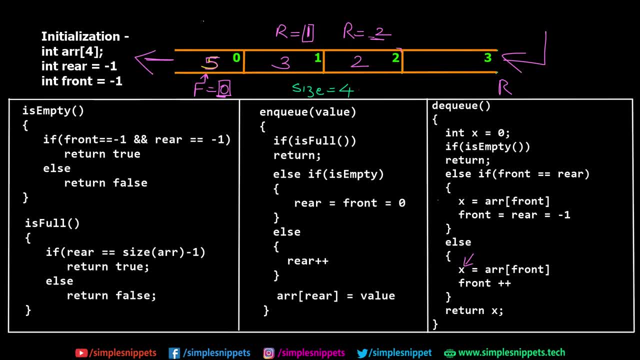 storing in x, i'm saying front plus plus, which means now front is also going to be incremented. so when i say f plus plus, f becomes one right. so now f is pointing the second location in the array and this has become, or this has removed, this has been removed from the q. now when i say 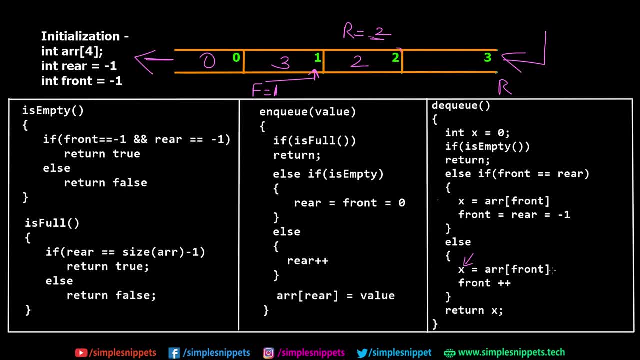 removed. what we can do is we can make it zero, also over here, arr of front equals to zero, and then we can do front plus plus. that's what we'll do in the coding part, but essentially what we are doing is we are incrementing the front variable by one. okay, so this is one dq operation let's do. 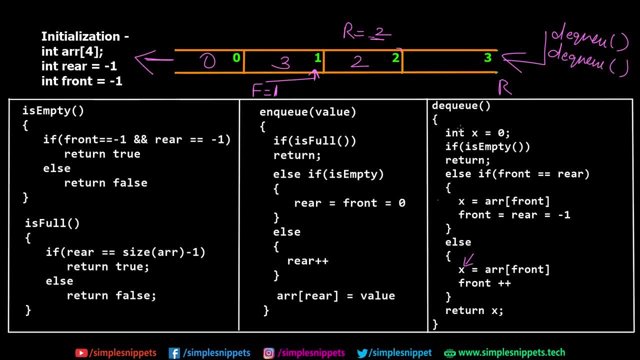 more dq operation. so i'm going to say dq again. what is going to happen? it is going to check for is empty. it's not empty because we have three and two still. r is pointing over here, f is pointing over here. that is, f is having this index value, r is having this index value. again, we are checking. 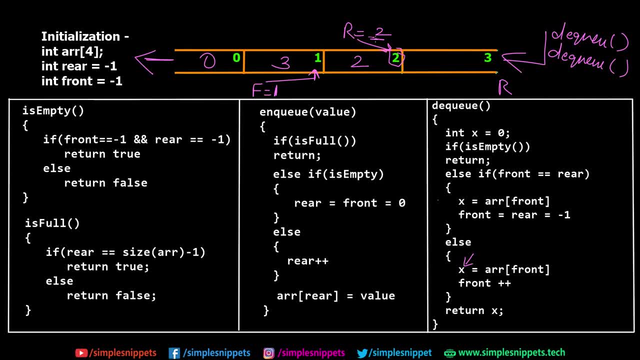 for if front and rear are equal, that is also not equal. f is one and r is two, which means what will happen is again the value at the front, that is, arr of front. arr of front is arr of one, which is three, is going to be dq'd. 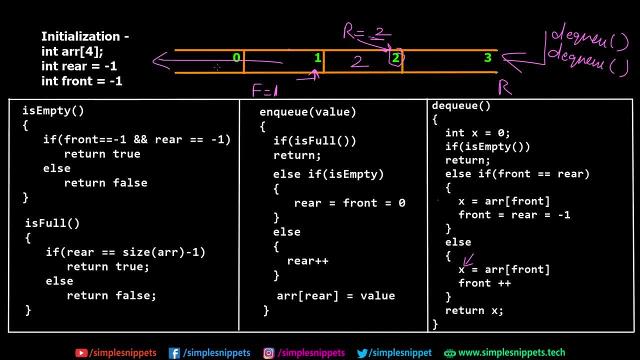 right, it is going to be removed. even this is removed. when i say remove, it can be made zero programmatically. and then we are saying front plus plus. so now front will be f equals to two. right, this is what it would be pointing. so if you perform one more dq operation, what will happen is 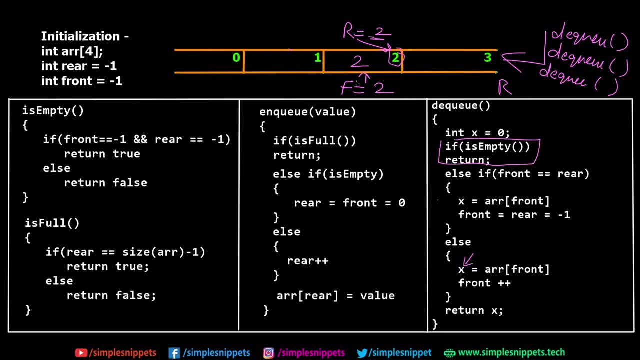 here of course it is not empty, because f and r are two and two. but now else? if operation is going to be executed, because front is equal to rear, both are storing value two. that is the second index. so what we will do is we will say x equals to arr of front, and now we are going to make front and rear. 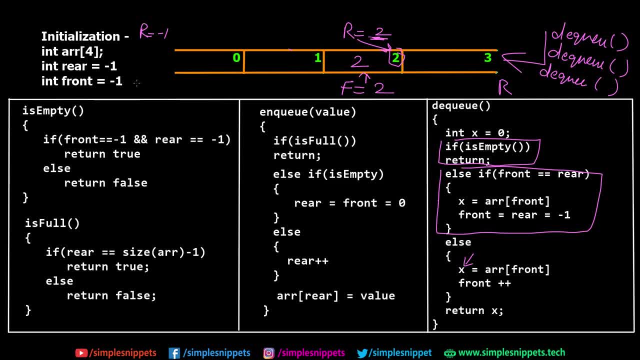 equal to minus one, so r will equal to be minus one, f will become minus one. so this is that minus one location, the invalid location that we have assigned as the empty condition. right? so this is what we are doing over here, because after moving this two from the q, we are left with no values, which means 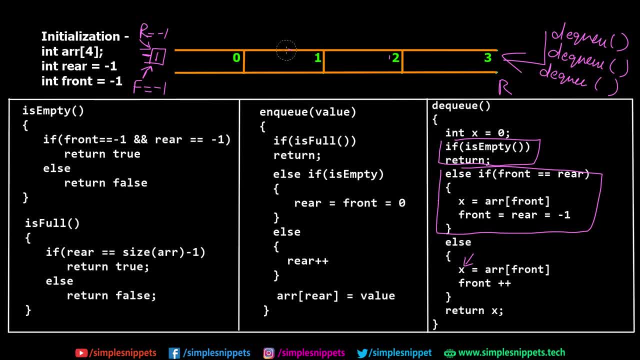 that the q is again become empty, so we can again start nqing values. right, so here's where else? if so, this is the nq and dq operation when it comes to a simple q data structure. now there is one drawback of this simple q data structure is because whenever you nq, you keep on incrementing. 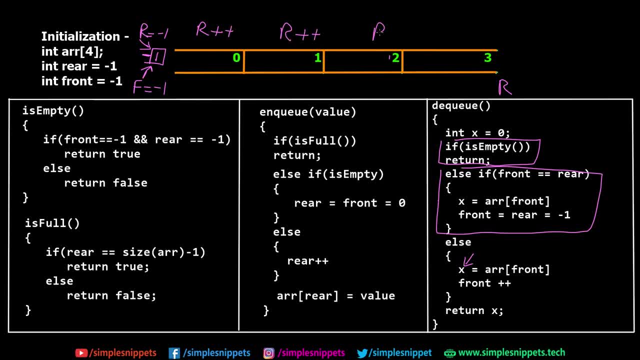 the rear. so you go r plus plus r plus plus, r plus plus, okay. and when you dq you keep on saying f plus plus, also right. so values go in like this: five, two, one, six, okay. and when they are removed they go in like this: and there comes a point where the left most values are unused. these values go. 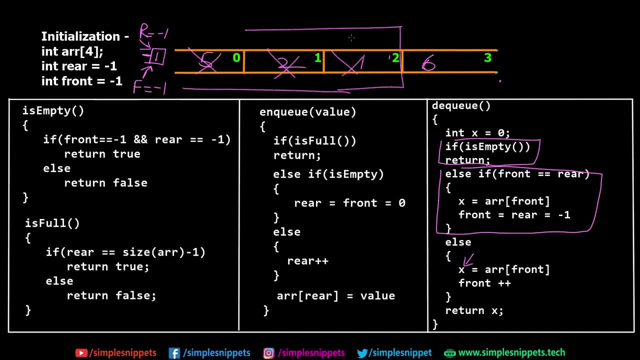 unused, because the rear pointer and front pointer are always incremented in this way, that is, in the opposite way through which the values are inserted, so that problem can be solved when we actually use circular q- and we'll discuss circular q in some other video, but i'm just trying to say that 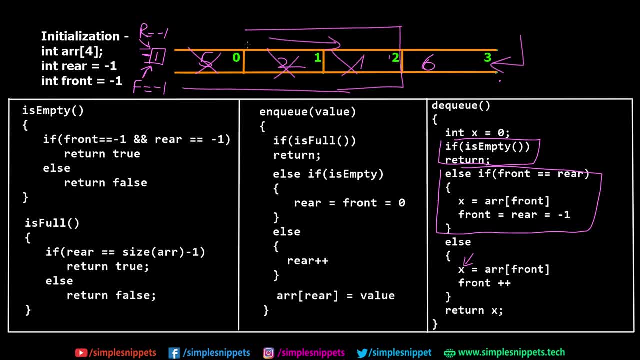 there are multiple ways in which q data structure can be implemented and there are different types also. so, yeah, these were the basic implementations of the q data structure and we will see you in the next part of q data structure and the standard operations that that are: is empty, is full nq and. 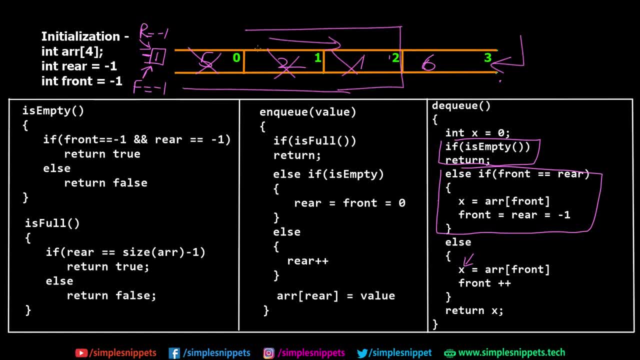 dq. there is one more, that is count. we will directly see it in program because that is very basic. you simply take the difference between the rear and the front value and you add one to it and that will give you the count. okay, so that's, that's just the basic thing. now one last thing that is left.